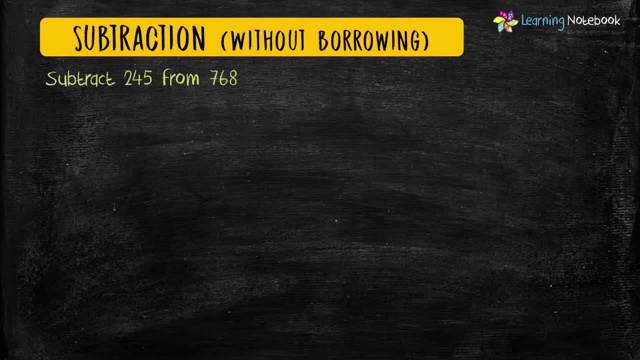 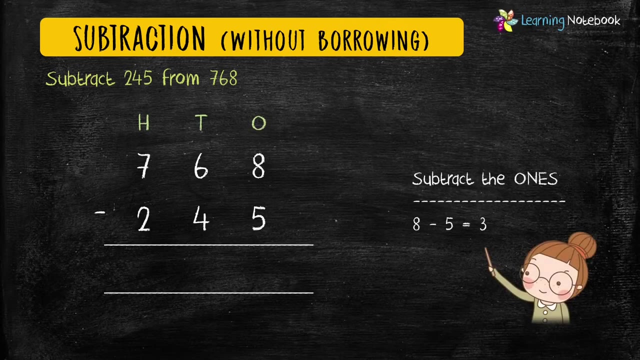 Question is: subtract 245 from 768.. To subtract these numbers, write them in column form. First, subtract the digits at 1s place: 8 minus 5 equals to 3.. Next, subtract the digits at 10s place: 6 minus 4 equals to 2.. 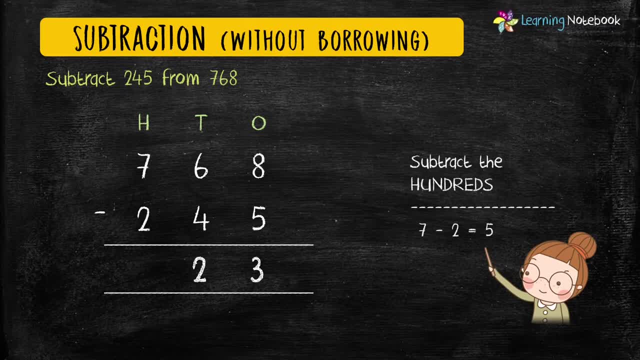 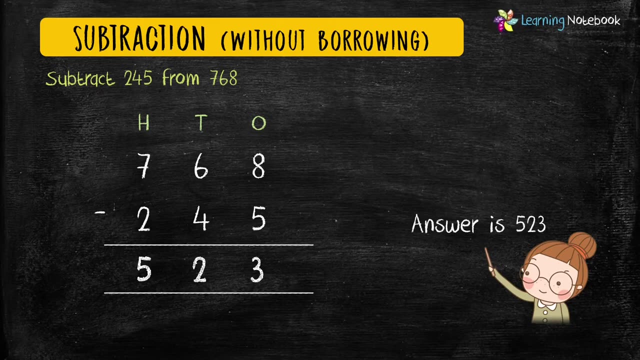 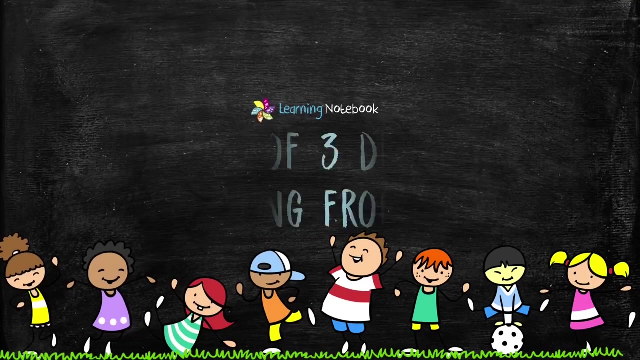 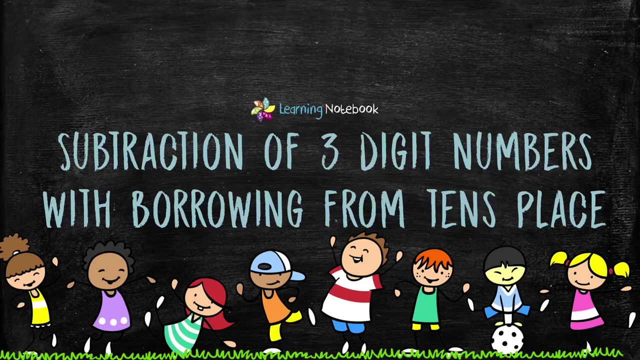 And next subtract the digits at 100s place. 7 minus 2 equals to 5.. So our answer is 523.. So, students, this is how we do subtraction of 3 digit numbers without borrowing. Now let's learn subtraction of 3 digit numbers with borrowing from 10s place. 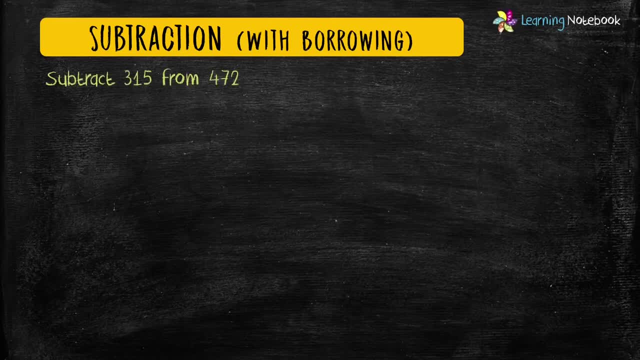 Question is: subtract 315 from 472.. To subtract these numbers, let's write them in columns. Question is: subtract 315 from 472.. To subtract these numbers, let's write them in columns. First, subtract the digits at 1s place, But 5 is a bigger number than 2.. 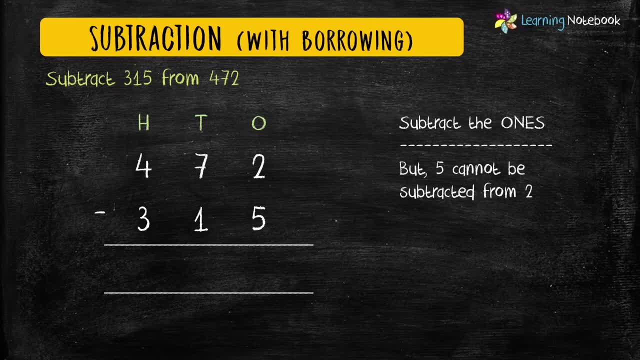 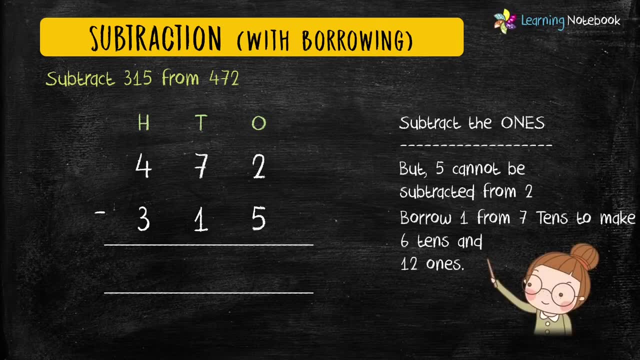 But 5 is a bigger number than 2.. So 5 cannot be subtracted from 2.. So we will borrow 1 from 7.. Therefore 7 becomes 6 and 2 becomes 12.. So we will borrow 1 from 7.. Therefore 7 becomes 6 and 2 becomes 12.. 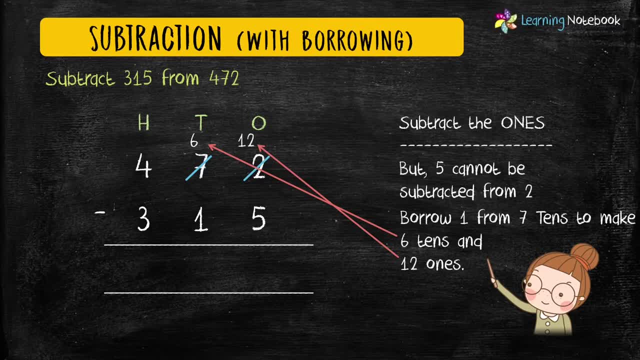 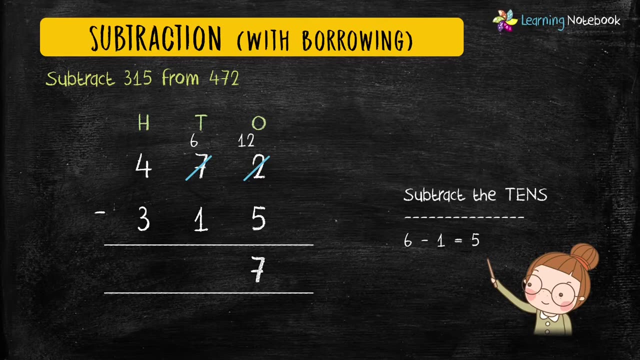 Now let's subtract digits at 1s place. Now let's subtract digits at 1s place: 12 minus 5 equals to 7.. Subtract the digits at 10's place: 6 minus 1 equals to 5.. 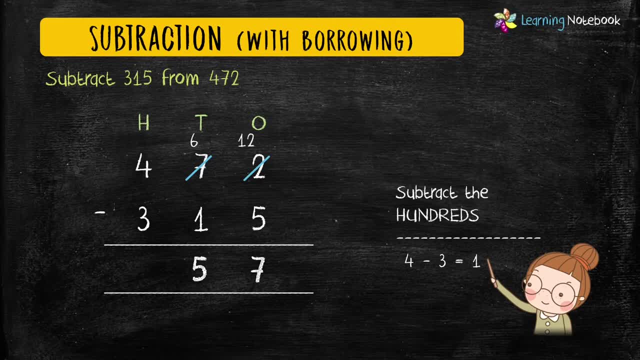 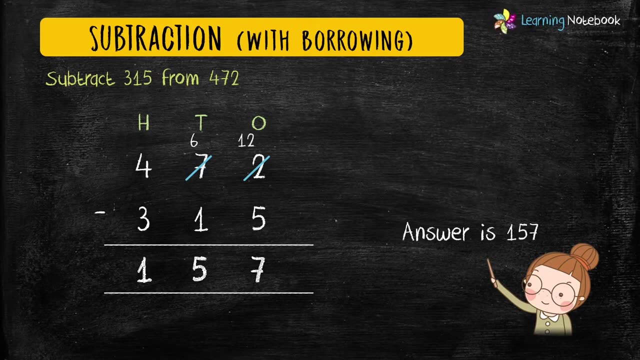 And next let's subtract the digits at 100's place: 4 minus 3 equals to 1.. So we get the answer as 157.. So, students, this is how we do subtraction of 3-digit numbers, with borrowing at 10's place. 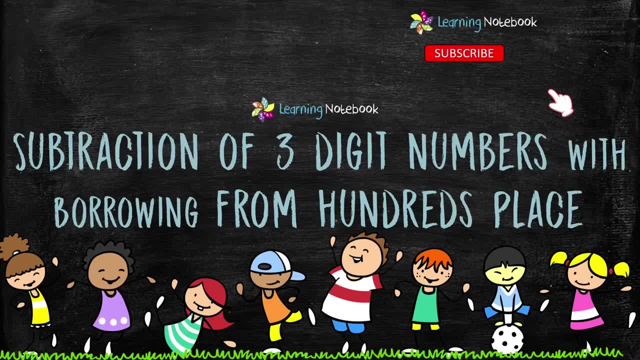 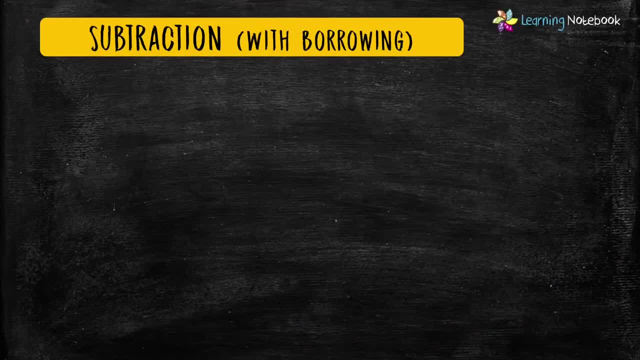 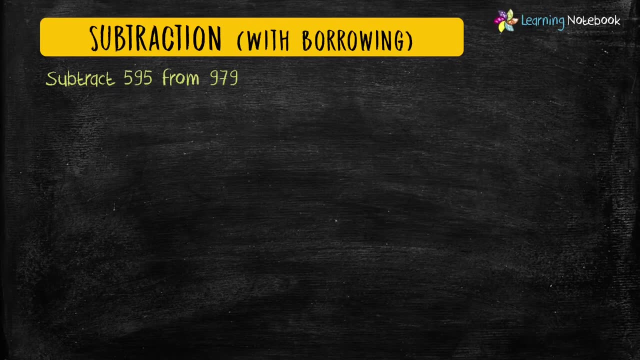 Now let's learn subtraction of 3-digit numbers with borrowing from 100's place. Question is: subtract 595 from 917.. Again, to subtract these 3-digit numbers, we will first write them in column form. Now let's subtract the digits at 1's place. 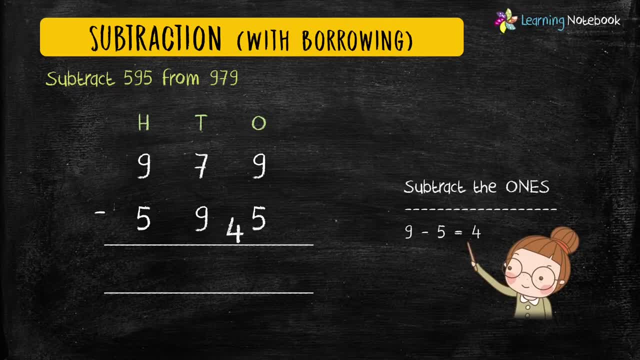 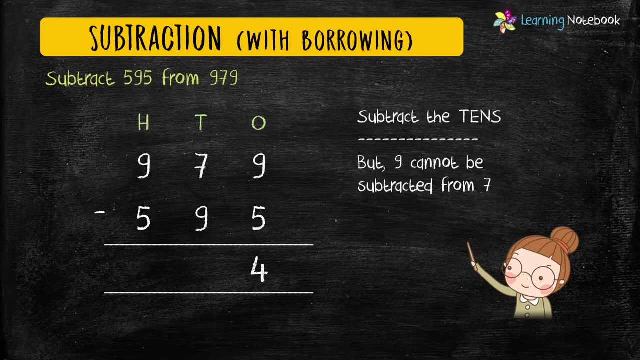 9 minus 5 equals to 4.. Now let's move and subtract the digits at 10's place. 9 is a bigger number than 7.. So 9 cannot be subtracted. So we will borrow 1 from 9.. 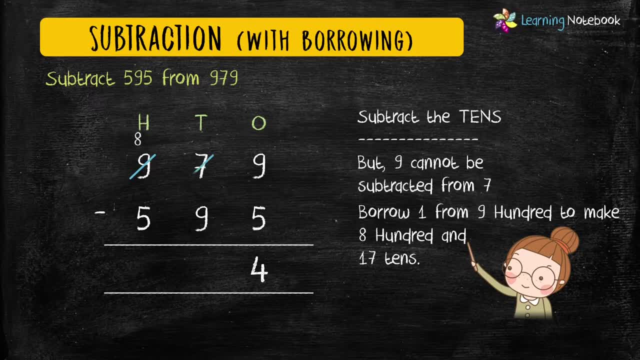 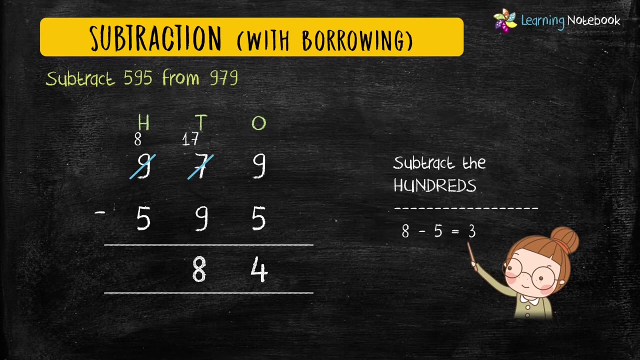 Therefore, 9 becomes 8. And 7 becomes 17.. Now we can subtract the digits at 10's place: 17 minus 9 equals to 8.. And next, subtract the digits at 100's place: 8 minus 5 equals to 3.. 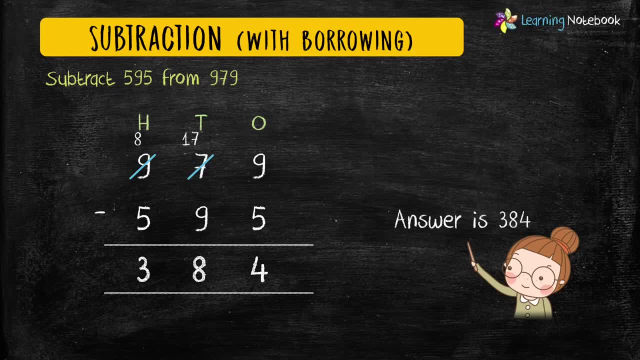 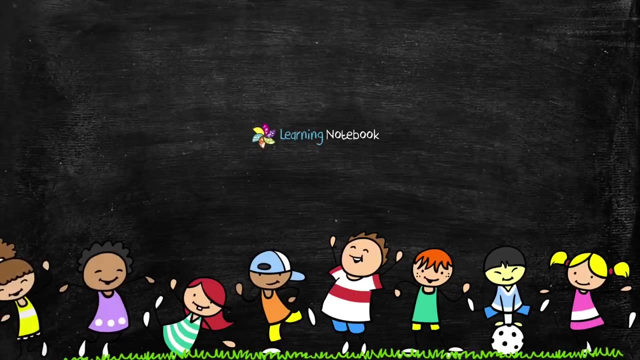 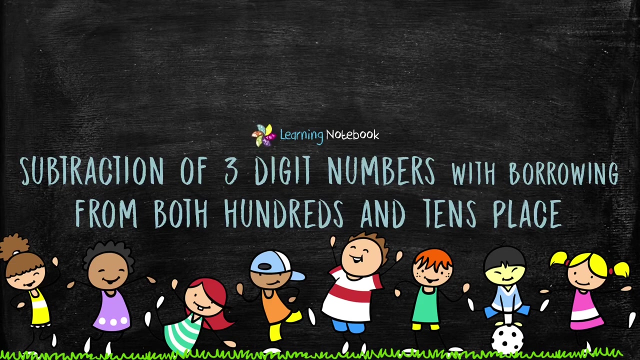 So we get the answer as 384.. So, students, this is how we do subtraction of 3-digit numbers with borrowing from 100's place. Now let's learn subtraction of 3-digit numbers with borrowing from both 100's and 20's. 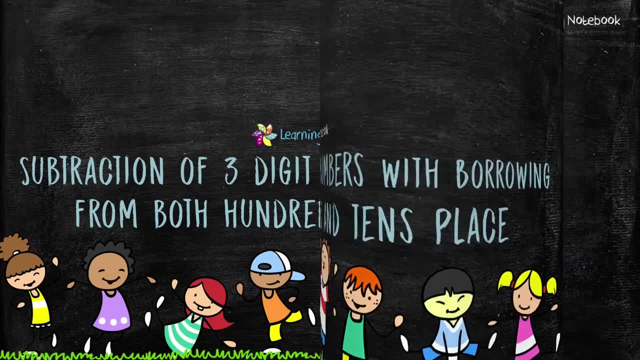 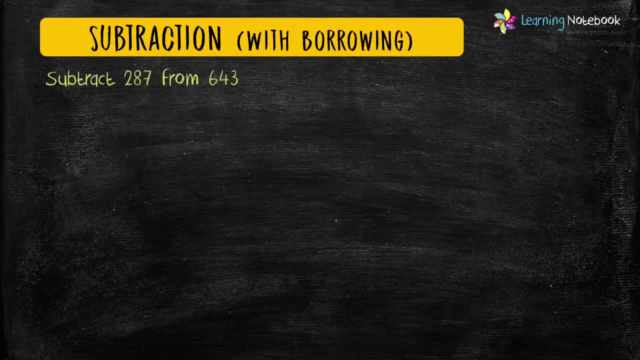 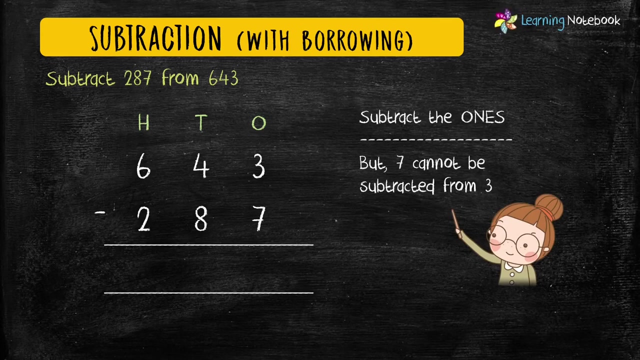 10's place. Question is: subtract 287 from 643.. Let's write the numbers in columns. Let's subtract the digits at 1's place, But 7 is a bigger number than 3.. So 7 cannot be subtracted. 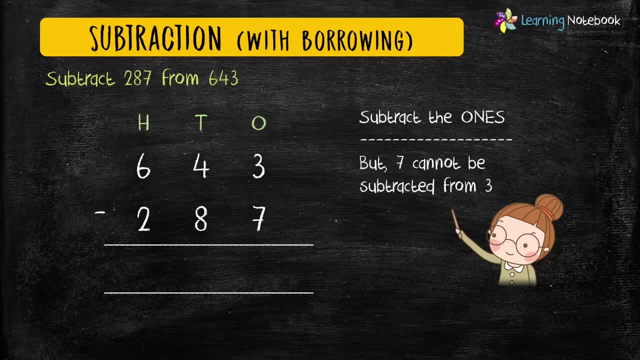 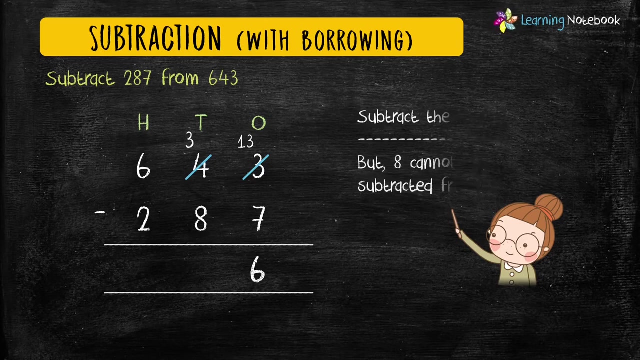 from 3.. So we will borrow 1 from 4.. Therefore, 4 becomes 3 and 3 becomes 13.. Now we can subtract 7 from 13 and we get 6.. Now let's subtract the digits at 10's place, But again 8 is. 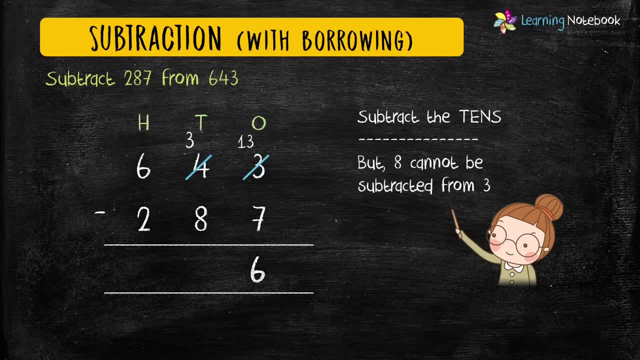 a bigger number than 3. So 8 cannot be subtracted from 3.. So again we will borrow, but this time we will borrow from 100's place, which is 6.. So 6 becomes 5 and 3 becomes 13.. Now we can subtract 8. 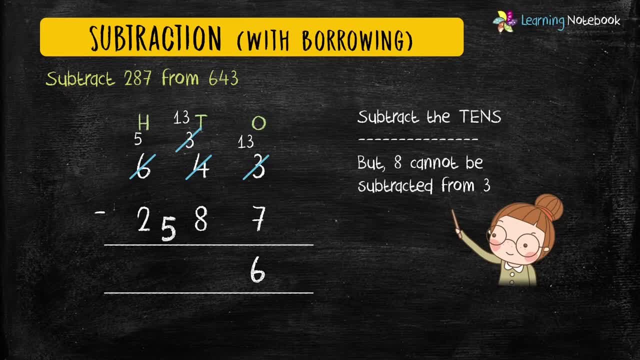 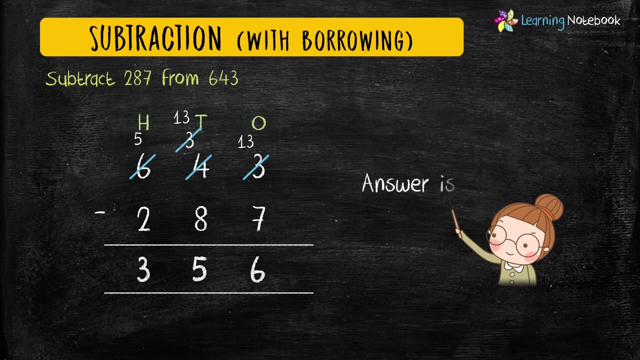 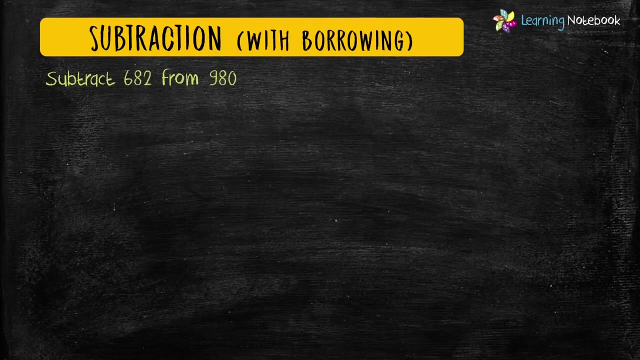 from 13 and we get 5.. Now let's subtract the digits at 100's place: 5 minus 2 equals to 3.. So our answer is 356.. Now, students, let's do one more example to understand. this Question is subtract 682. 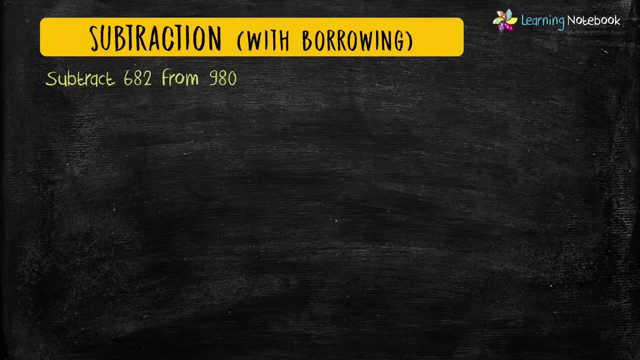 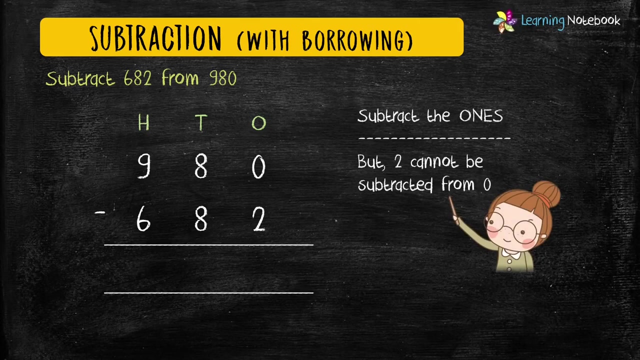 from 906. 80.. Let's first write these numbers in columns. Now let's subtract the digits at 1's place. But 2 is a bigger number than 0. So 2 cannot be subtracted from 0. So we will borrow 1. 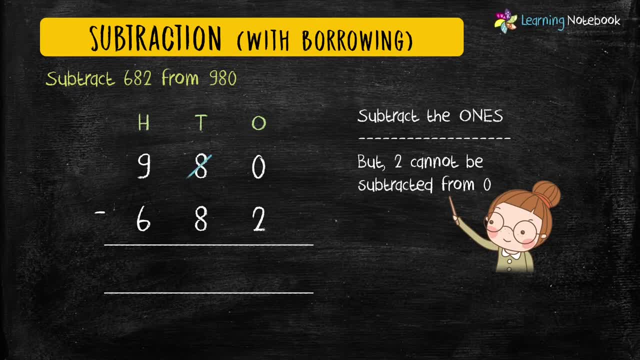 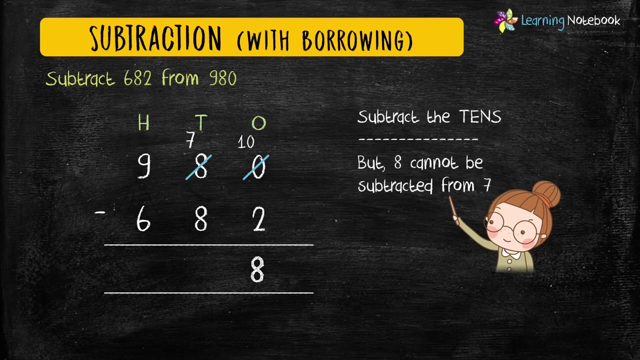 from 10's place which 8 is. So 8 becomes 7 and 0 becomes 10.. Now let's do the subtraction 10 – 2 equals to 8.. Now let's subtract the digits at 10's place. But 8 is a bigger number than 7.. So 8 cannot. 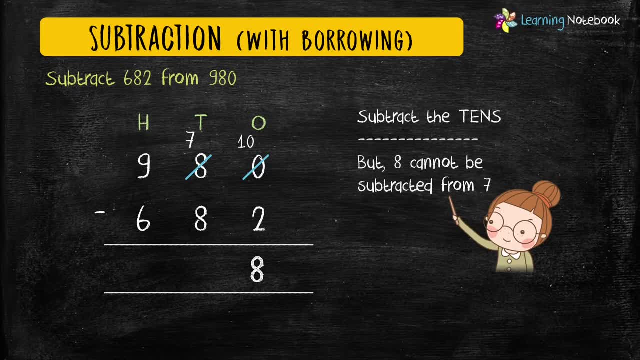 be subtracted from 10's place, So 2 cannot be subtracted from 10's place, So 8 cannot be subtracted from 7.. So let's borrow. We will borrow from 100's place, So 9 becomes. 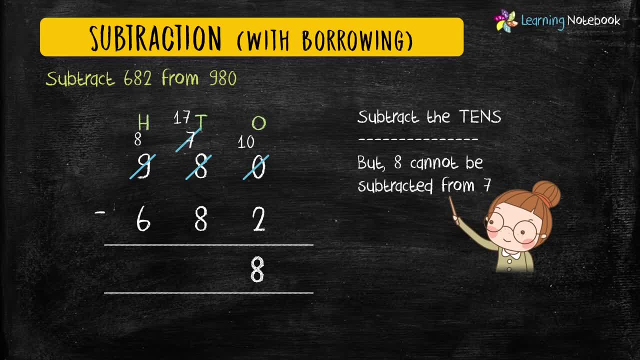 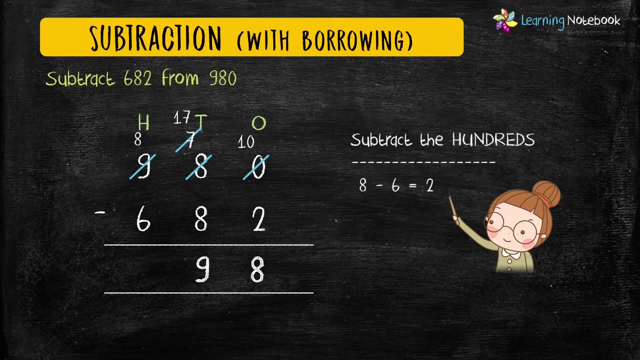 8 and 7 becomes 17.. Now we can easily subtract 8 from 17 and we get 9.. In the end, let's subtract the digits at 100's place. 8 minus 6 equals to 2. So we get the answer as 298.. 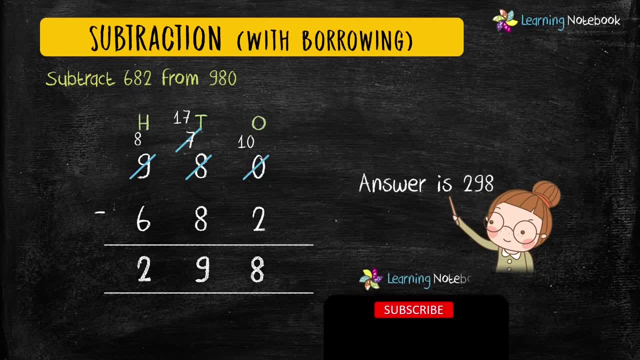 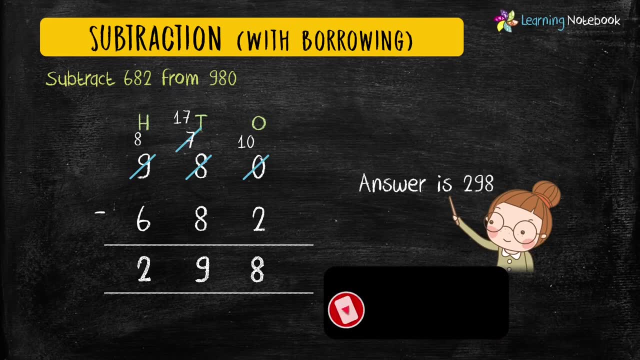 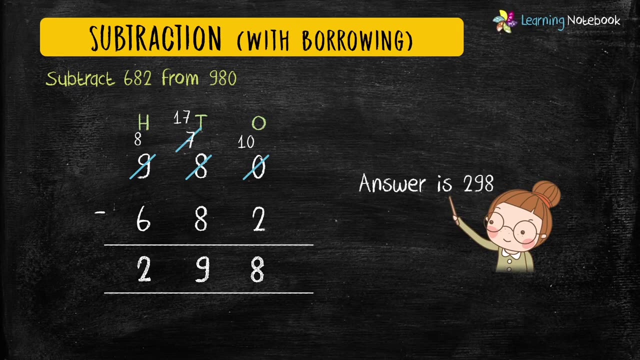 So, students, now I am sure you have understood how to do subtraction of 3 digit numbers with borrowing. We have got many amazing worksheets and interesting quizzes on math. That's for class 3 on our channel Learning Notebook, So do visit our channel. Thanks for watching.